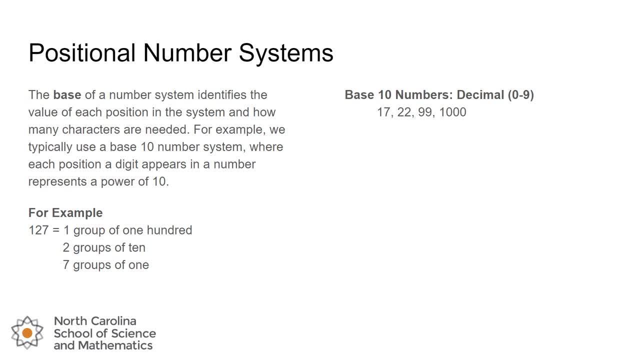 We are most familiar with base 10 numbers, so we would call that decimal and there's a couple of examples there: 17,, 22,, 99,, 1000.. And again, decimal uses the numbers 0 through 9.. 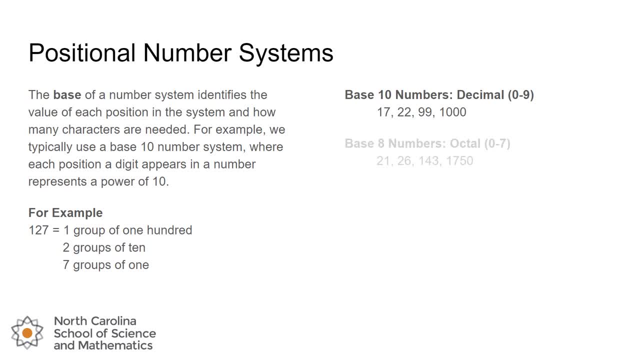 Now we're going to represent those same exact four quantities using different bases. So another commonly used base in computer programming is octal. So, as you might see from both the name and the base number, octal is a base of 8, and. 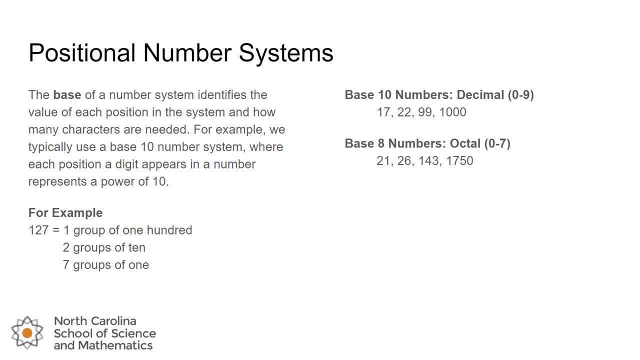 it uses the characters 0 through 7.. So the number 17 in base 10 becomes the number 21. We might read that as 21,, because our brain is so trained on decimal, But the characters 2,, 1, and base 8 is still 17.. 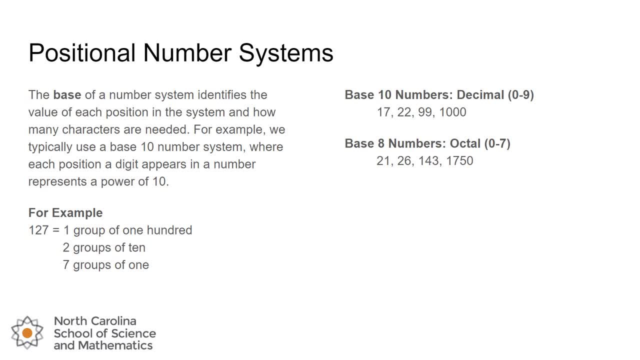 So it gets a little confusing when we're working on other bases. when we try and read them out loud, The number 22 in decimal becomes the number 26 in octal- Same quantity, even though they look different- And so on down the line. 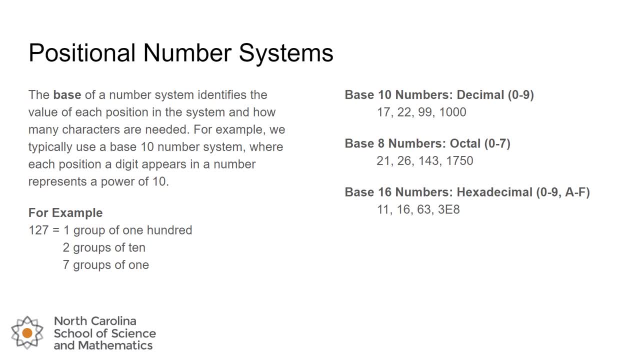 Another common representation of numbers in computer programming is hexadecimal, so base 16.. And our characters for that? this is where it gets a little tricky, unlike octal where we reduce the number of characters, so we just don't use 8 and 9, hexadecimal needs. 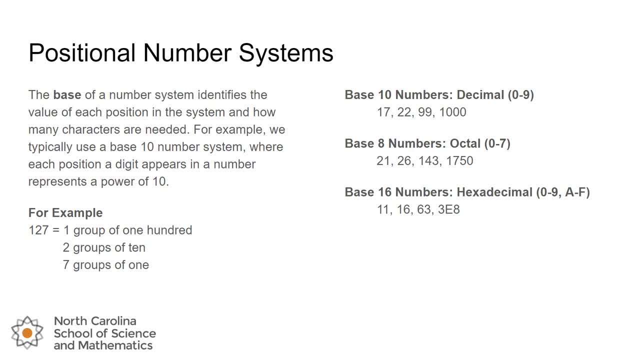 more characters. So we're going to go 0 through 9, like normal, but when we get to our 10th character out of the 16 that we need, we're going to switch over to the alphabet. So a quantity of 10 will be represented by a. a quantity of 11 will be represented by. 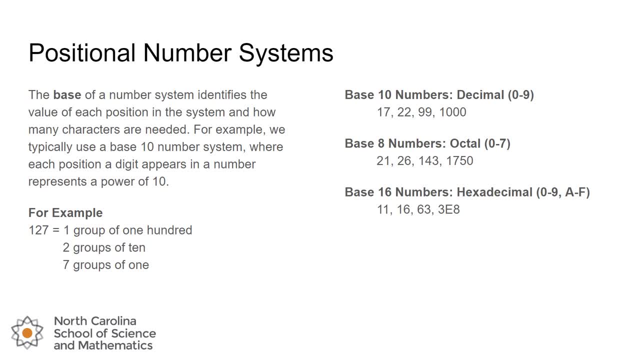 b all the way up to a quantity of 15 represented by the letter f. So while we might say 17 in base 10, that's 1, 1 in hexadecimal. 1000 in decimal is 3e8 in hexadecimal. 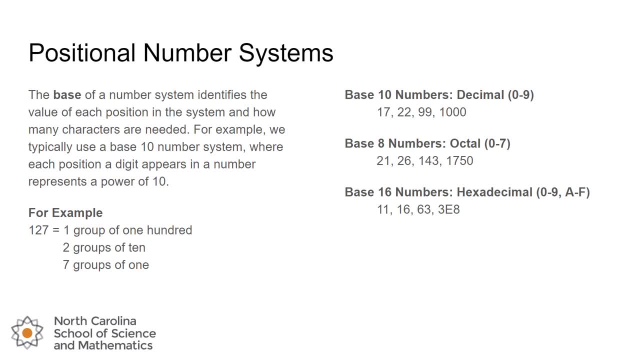 And we're going to talk in just a second about how we can convert back and forth between these, so you don't have to worry about that quite yet. And then, probably the most commonly known alternate base number system that's used in computer programming is binary. 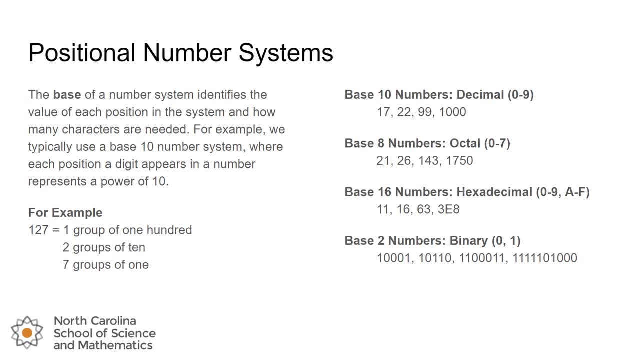 Only two numbers, So we just use the numbers 0 and 1.. So the number 17 in base 10 becomes 1, 0, 0, 0, 1.. And the number 1000 becomes 1, 1, 1, 1, 1, 0, 1, 0, 0, 0. 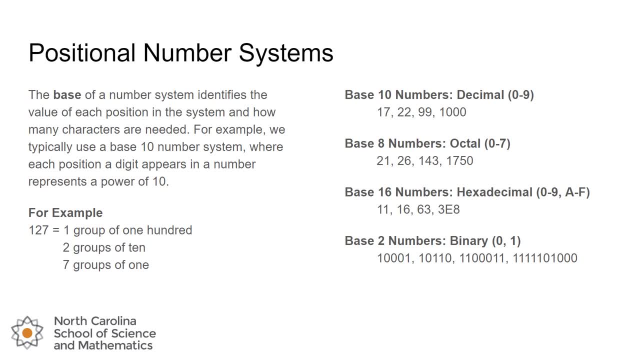 And again, we're going to talk about that later. Okay, We'll talk about how to convert over to that in just a moment, But these are the ones you're going to want to be familiar with when we're working with cryptography and programming, because different types of ciphers when we start using computers. 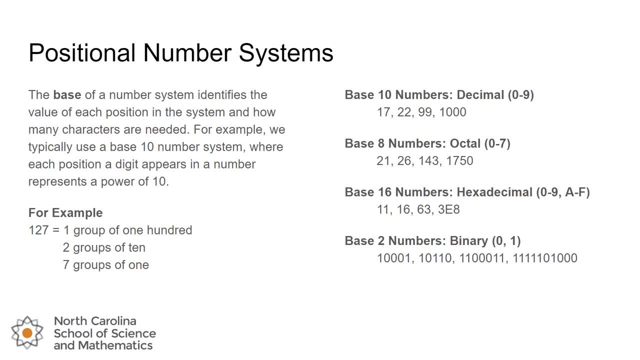 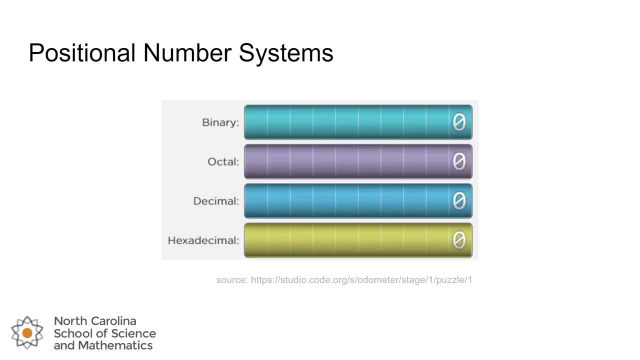 might implement operations in different bases- And that'll be a lesson that we'll cover in just a little bit- is how do we do mathematical operations with these different representations of the numbers? Here's a nice visual that kind of shows you counting in the different number systems. 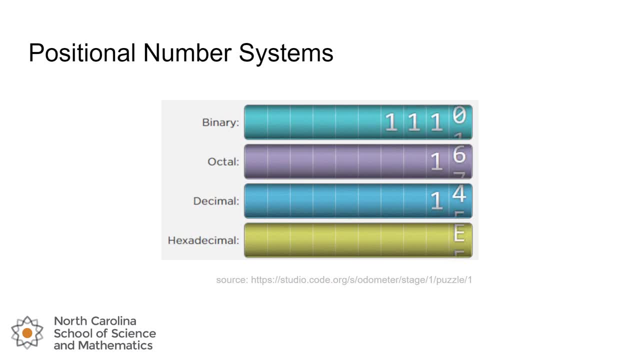 so the the, The third row labeled decimal in the blue, is counting, probably like we are used to counting, but we can see the counting taking place in the alternate number systems as well. So you can see that kind of binary is growing the fastest, octal kind of somewhere in the. 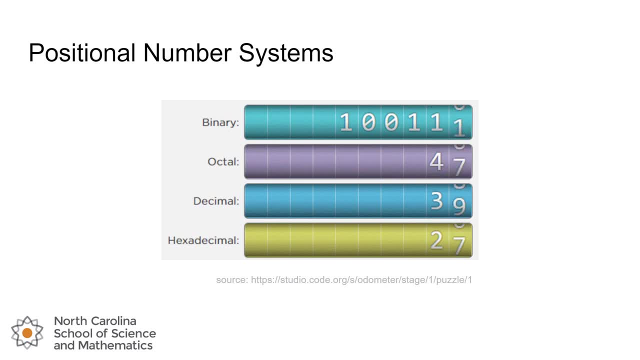 middle with decimal and then hexadecimal. if we let this run for just a little bit, we'll see continues to grow, but we need fewer characters. That's part of the reason why people like hexadecimal is that it requires fewer characters or fewer positions, rather to represent the same size number. so we can see that hexadecimal. 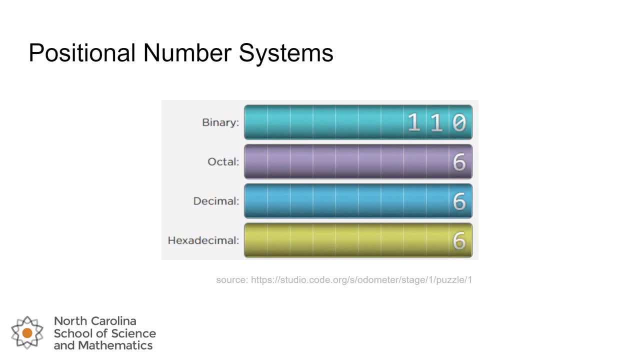 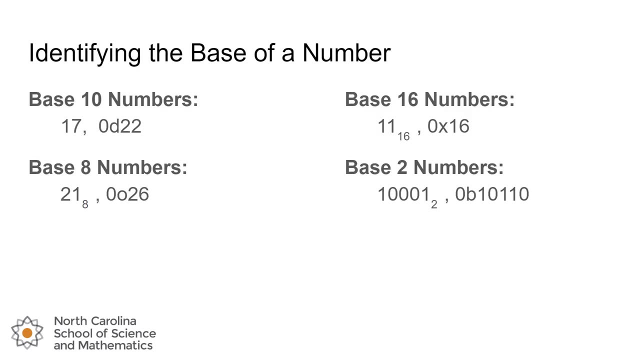 got up to like five something. only two places used where binary had like eight in there. So it's a little more compact way to write especially large numbers, Because it's not always obvious which base our number is going to be in when we write. 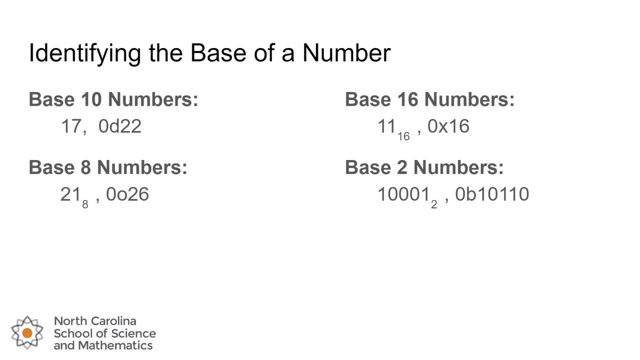 down the characters, like three and then a seven, like: is that three, seven, thirty-seven, Or is that three, seven as a base eight number or a base sixteen number? So these are some conventions that you'll see, depending on the context. 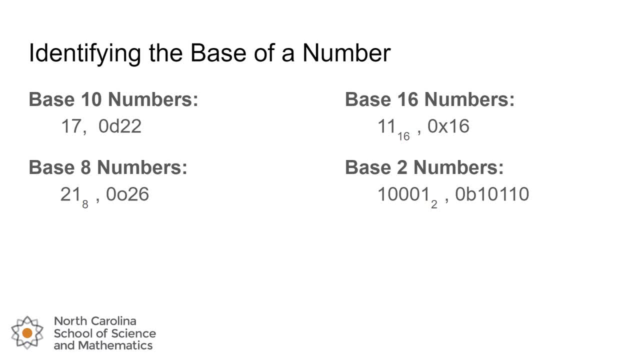 So base ten numbers. you would just write seventeen, one, seven. no additional information needed If you wanted to write the number twenty-two in base ten. another way we could do that which is common when you're programming, is the prefix zero and then the lower case letter. 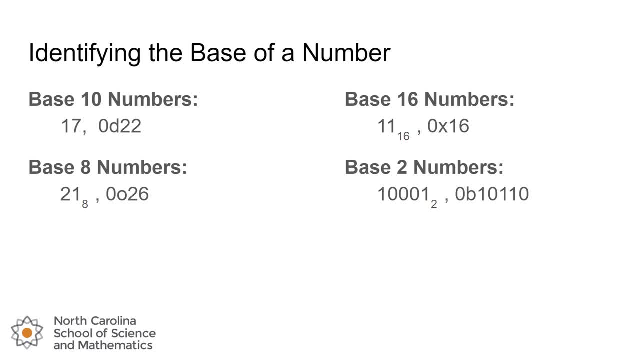 d to represent decimal, and then you just write the number after the d Base eight. the number seventeen would be two, one, and then a subscript of eight, and then likewise the number twenty-two. When we convert to octal it becomes two, six, and we can represent that with a zero and. 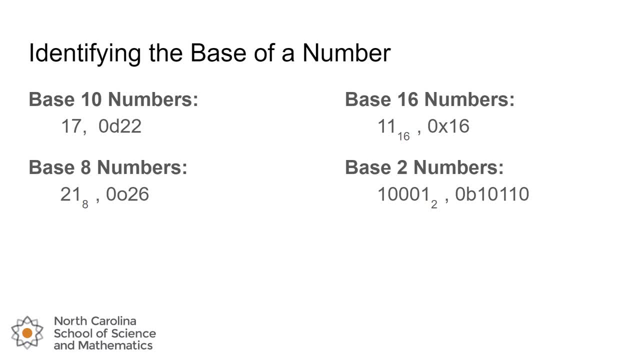 then a lower case o as the prefix. Similar types of notation: for base sixteen and base two you can use a subscript that denotes the base of the number that you've written with the characters, or: hexadecimal can have a prefix of zero x and binary will have a prefix of zero b. 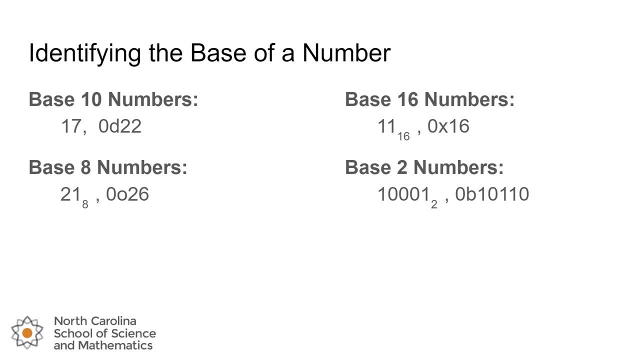 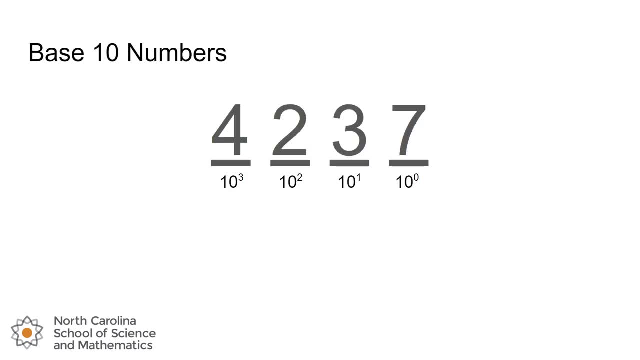 All right, let's take a look at actually doing some conversion of other bases into decimal. Let's just start with kind of a refresher how we take our normal base ten numbers and we convert them to a value in our head. So here we've got the number four thousand two hundred and thirty-seven four, two, three. 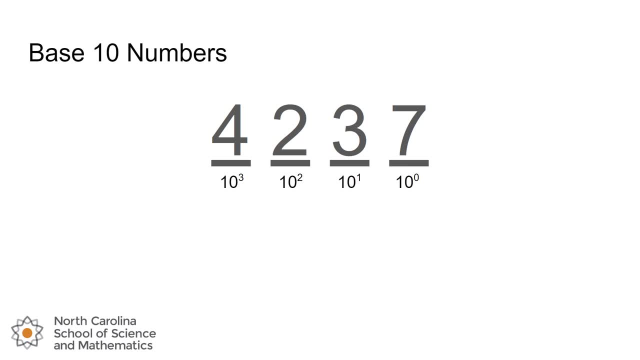 seven, and under each place I've written the value of that position. So the seven is ten to the zero. so again, that's seven ones Under the three, we've got ten to the one, which means we have three tens Under the two. we've got ten squared, so we've got two one's. 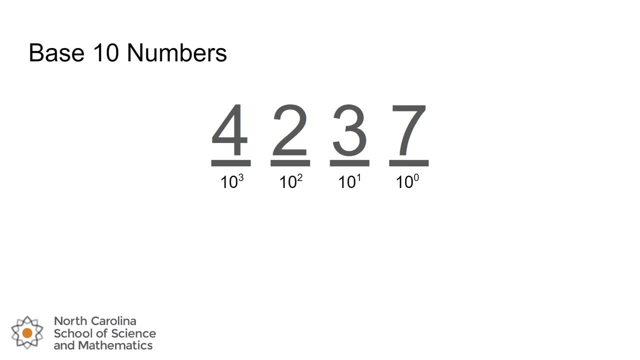 And then under the four we've got ten cubed. so that's four one thousands. We can kind of write it out like that: So four times ten to the cubed, plus two times ten squared, plus three times ten to the one, plus seven times ten to the zero, gives us the quantity that we're looking for here, as 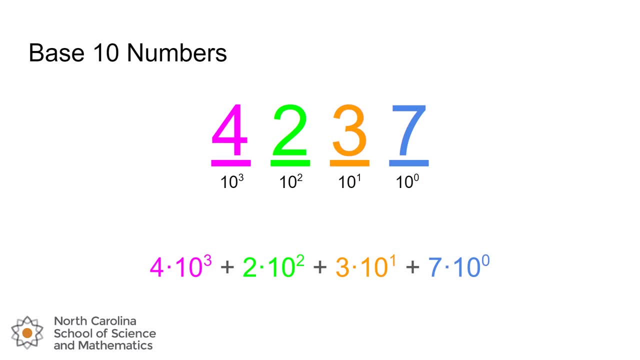 decimal. Now this one's already in decimal, so that doesn't really illuminate anything to us, but having that strategy is going to be helpful when we do work on other bases. So, for example, let's take a look at the binary number one zero one one. 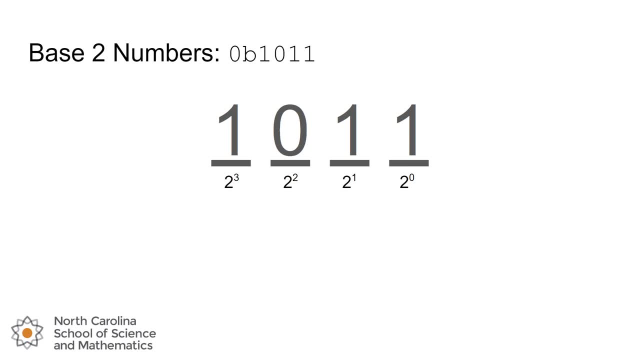 And say we wanted to figure out what that was. as a decimal, We can use the value of each position to help us convert. So, like we did before, we can kind of work from left to right. The first number one indicates to us that we have one group of two cubed, so one times. 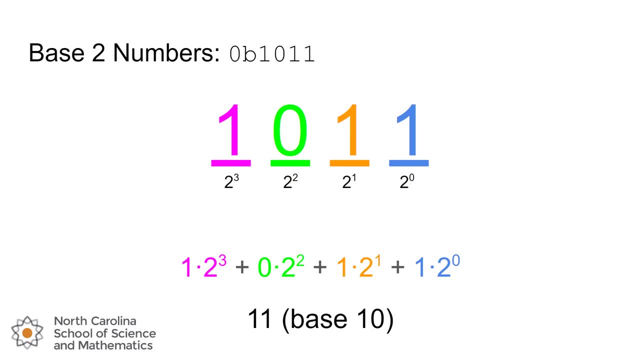 two cubed, that's eight plus zero of two squared. so we've got none of those. so that's going to add on zero. And then the orange one, So one, two to the one. We'll add that on. so now we've got eight plus zero plus two. 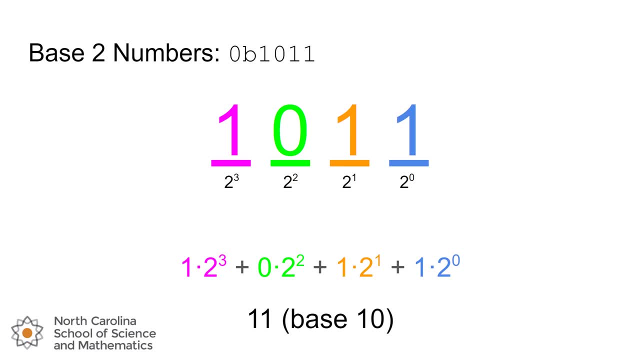 And the last one is one group of one, because two to the zero is one. So we add all that all up and we get eleven written as a base ten number. We can do the same thing with hexadecimal. Again, as a reminder, b is basically equivalent to the number eleven, whereas e is equivalent. 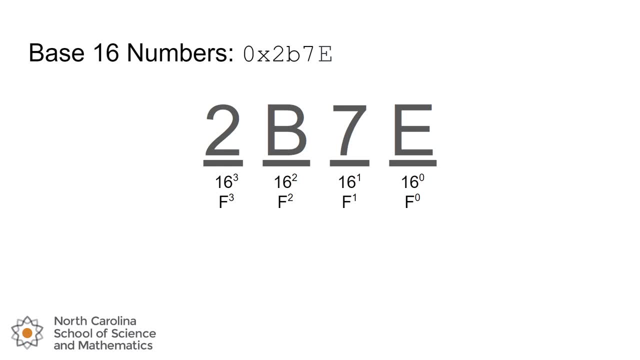 to the number fourteen. So that'll become helpful here In just a moment. So we're going to convert these to decimal by again same operation. So the number two tells us we have two groups of sixteen cubes. b tells us we have eleven. 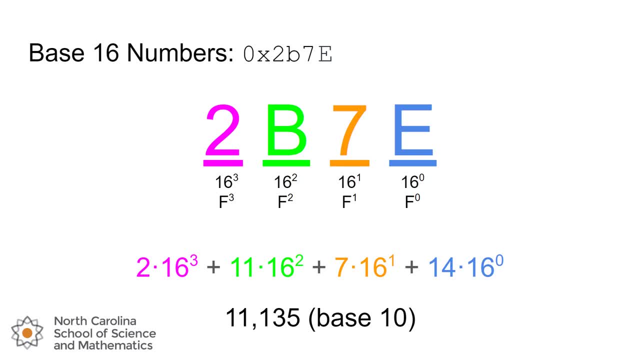 groups of sixteen squared seven tells us we have seven groups of sixteen to the one, and e tells us we've got fourteen groups of sixteen to the zero. So we can just throw that into a calculator and we'll crunch out the number eleven thousand. 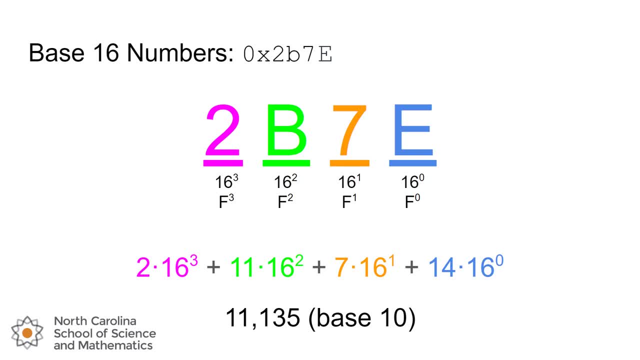 one hundred and thirty five. So again it's the same number, just two different ways to write it: Two b, seven, e, Hexadecimal eleven thousand one hundred and thirty five, base ten. Going the other way is a little bit trickier, but it's not too bad. 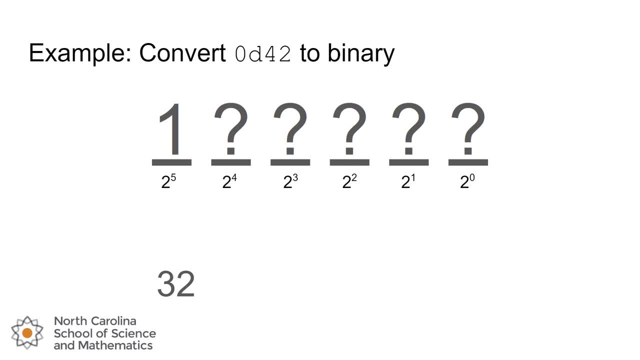 So let's convert decimal numbers to other bases. So let's say that we've got our binary number, sorry, our decimal number four two. we want to convert it to binary. So the first question is: what is the biggest power of two that is less than the number. 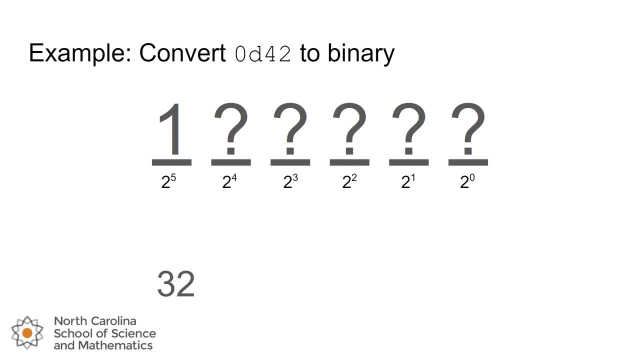 we're working with. So we know that two to the fifth is thirty two, And that is smaller than forty two. The next largest power of two, two to the sixth, is sixty four, And that's bigger than forty two. So we know that this number is going to be no bigger than two to the fifth. 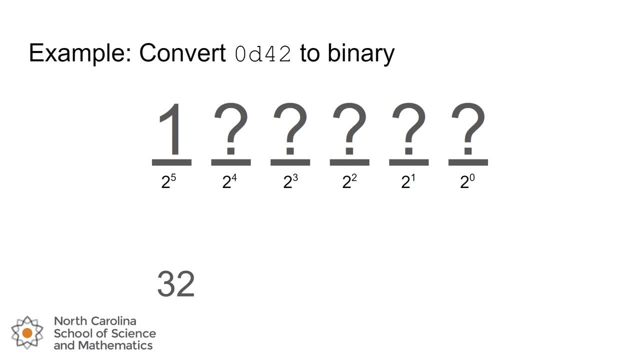 We know that this number will require no more digits than the one in the two to the fifth position. We call this number a six bit number and binary. each position is referred to as a bit, So two to the fifth is the largest bit that we need. 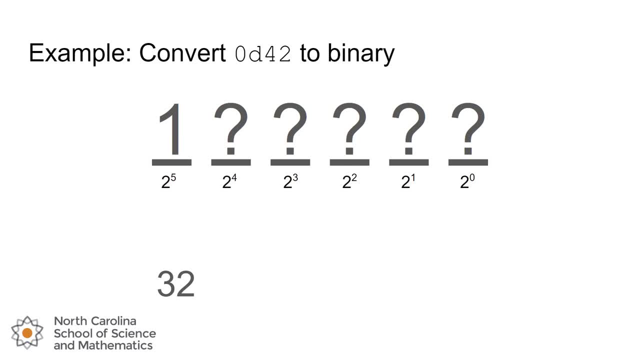 And we'll need no more than six bits to represent this number. So now that we know that the first position of the number is one in the two to the fifth position, we need to figure out the remaining bits, And we know that, in total, the remaining bits need to account for the last ten of value. 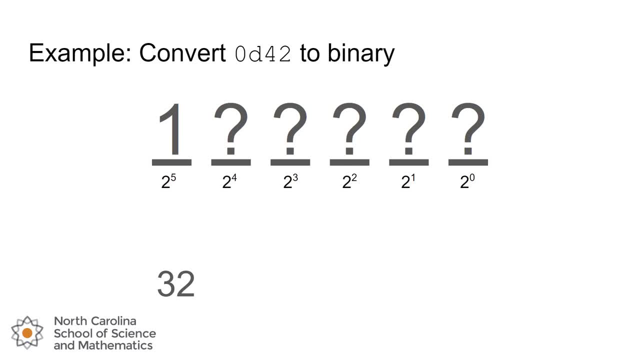 of forty two. That first bit accounts for thirty two out of the forty two. The remaining five bits have to account for the last ten. So we need to think about, okay, if I need to add ten more to the value here, what's. 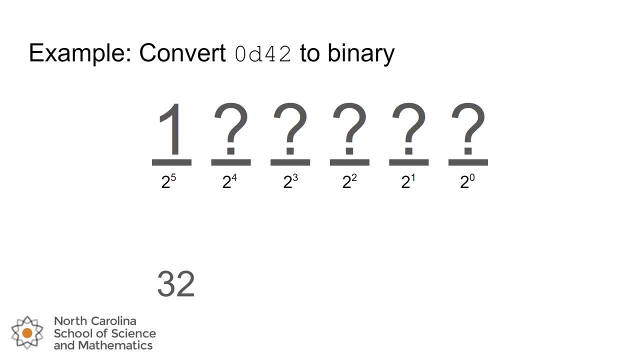 the next biggest power of two that is smaller than twenty, two That is smaller than ten And that's two cubed. So I'm going to start filling in some of these blanks here. I now know that from going from left to right, I need one zero one, and two to the fifth. 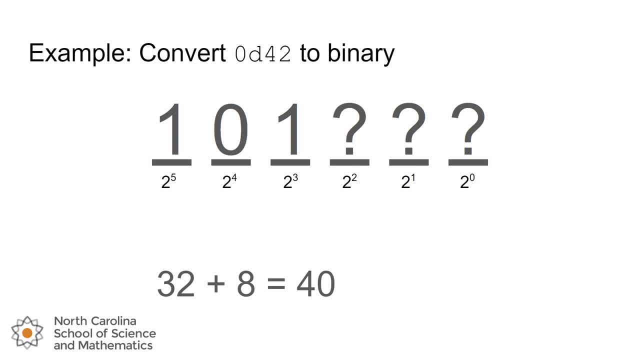 two to the fourth and two to the third respectively, And that gets me up to a total of forty. So I need to represent two more with the remaining three bits. Now, lucky for us, there's a position that represents a value of two, and that's the. 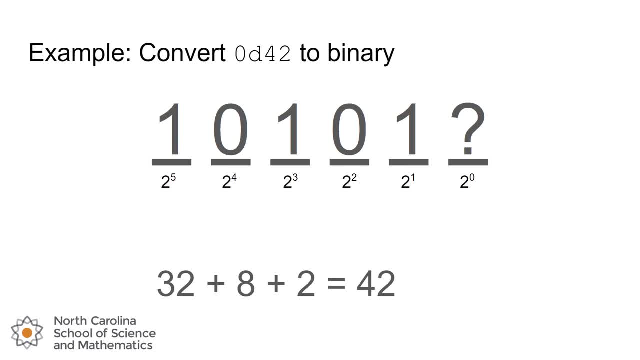 two to the one spot, so we can fill that up. And at this point the bits that we've written account for all of the value we need from this number. So that last spot must be a zero. So again we can verify a similar way that we just saw. 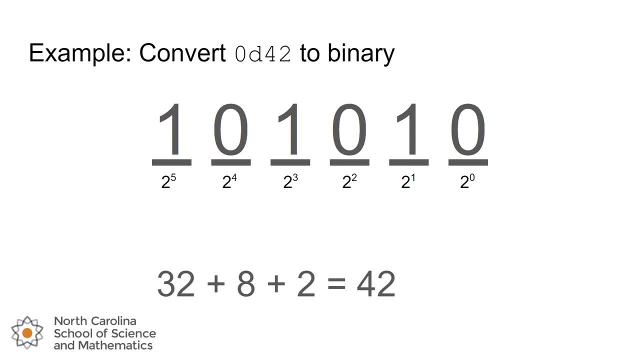 We have one group of two to the fifth, one group of two cubed and one group of two to the one. Together, those things are thirty two, eight and two, which totals up to forty two. We can do the same thing with hexadecimal. 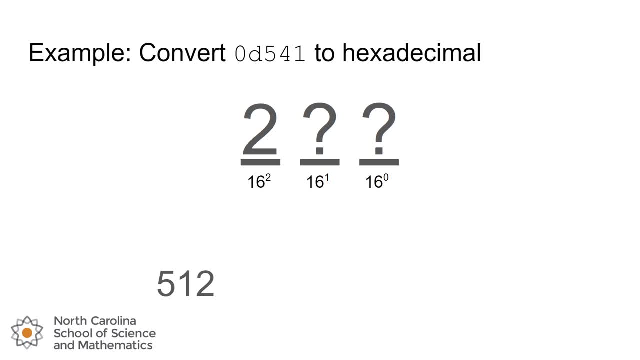 So if we have the decimal number five hundred and forty one, there are two groups of sixteen squared. Sixteen squared is two hundred and fifty six, So there's two groups of that that fit into five forty one, because that would be five hundred and twelve. 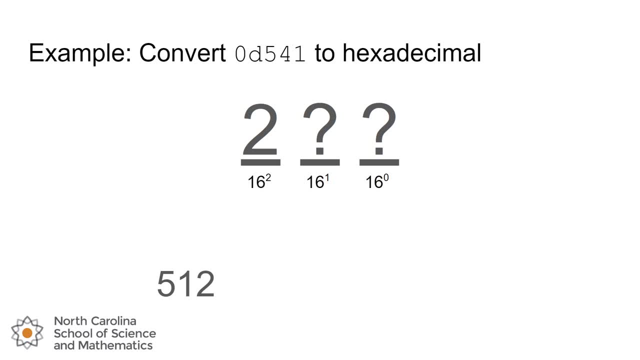 That means that we have a remaining value of twenty nine that we need to account for. So if we need twenty nine, I know I can do that with one group of sixteen. That gets me up to five hundred and twenty eight, And now we have a remaining thirteen that we need to account for. with the last position, 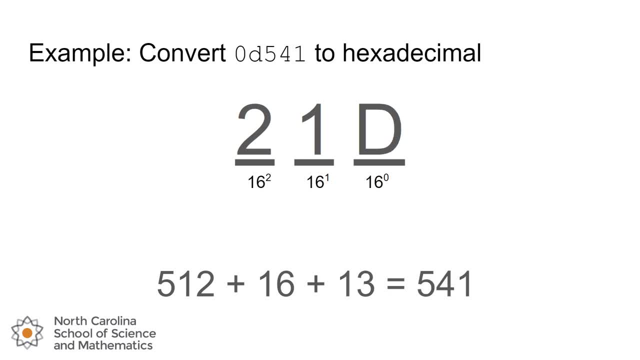 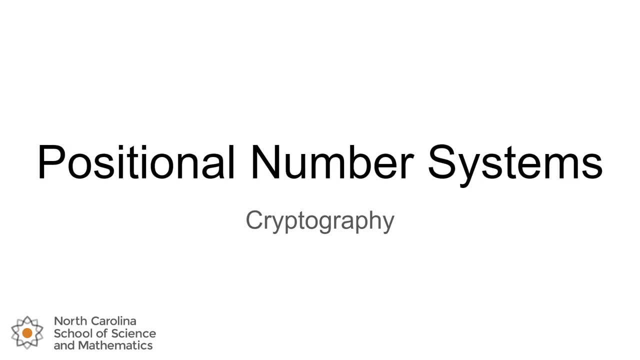 And thirteen has its own character in hexadecimal, It's the character d. So two one One d is equivalent to five hundred and forty one in decimal. So that's that's the quick version of what a positional number system gets you Multiple ways to represent the same number. 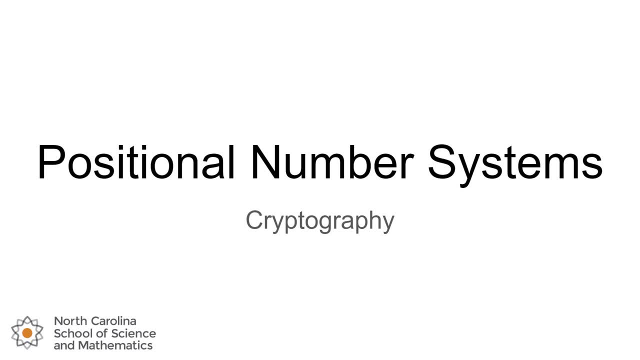 We can convert back and forth to decimal, and we could even- there's some algorithms for directly converting, say, from binary to hexadecimal or octal to binary. But for the purpose of this course, just going back to decimal and then decimal to your new,